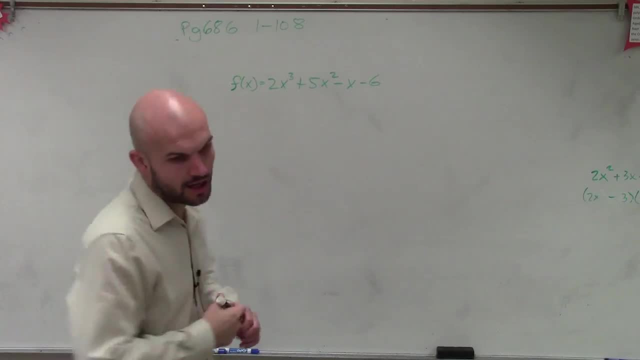 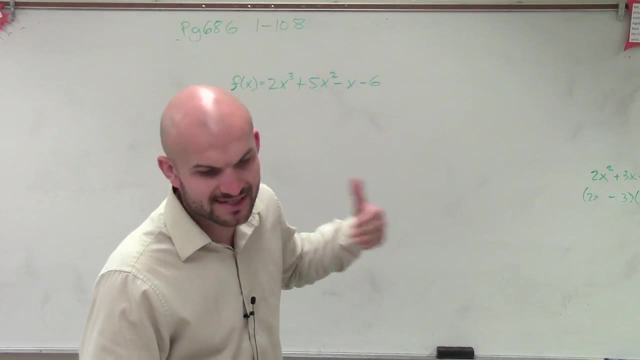 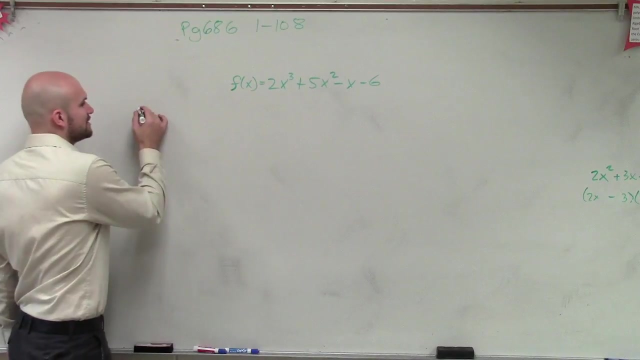 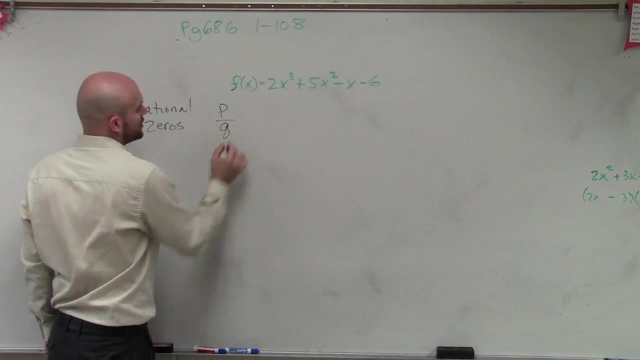 So I'll just show you guys what to do. First of all, what this question is asking us to do is, given the polynomial function, determine all the possible rational zeros and then state the rational zeros. So actually, with this one, we don't need to find any of them, We just need to state the rational zeros. So, remember, all of your rational zeros can be written as p over q, Right Where here's your p and your. 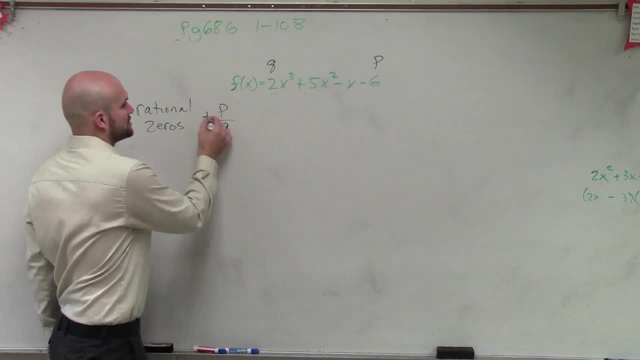 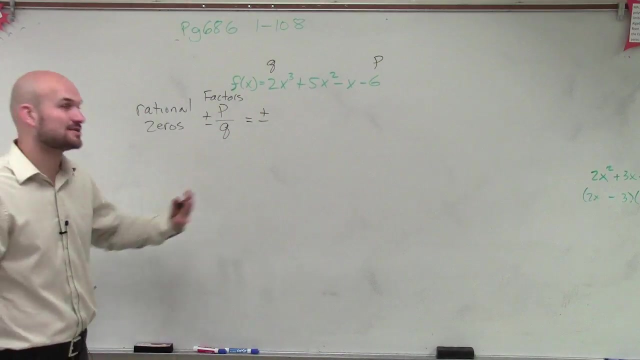 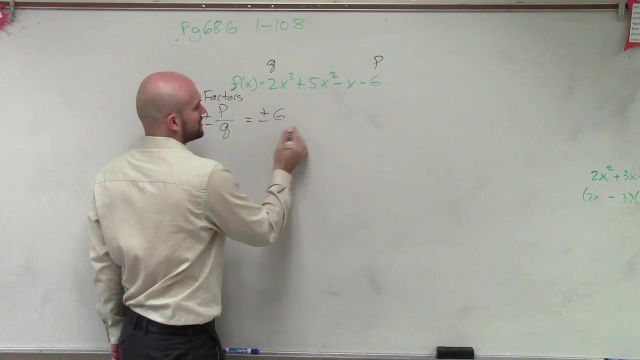 leading coefficient is your q. So remember, actually it's plus or minus. So therefore I simply have plus or minus. Now what I'm going to do, I'm sorry- rational zeros are the factors, sorry, are the factors of p over q. It's not just p over q, It's all the factors of p over q, So I can take out all the factors of 6.. So if I look at this, I could do 6.. So plus or minus 6, comma, plus or minus 3, comma, plus or minus 2,. 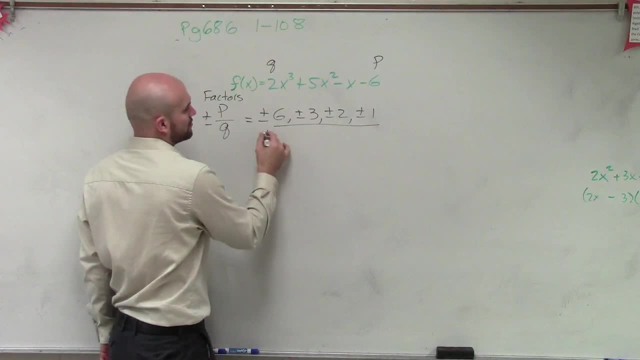 comma plus or minus 3, comma plus or minus 2.. plus or minus 1, over all the factors of 2, plus or minus 2, comma plus or minus 1.. What if you get P as 2?? 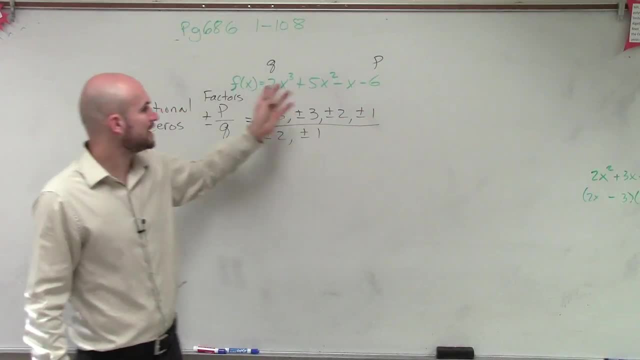 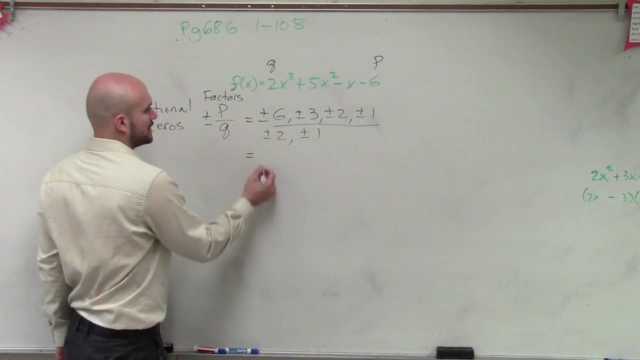 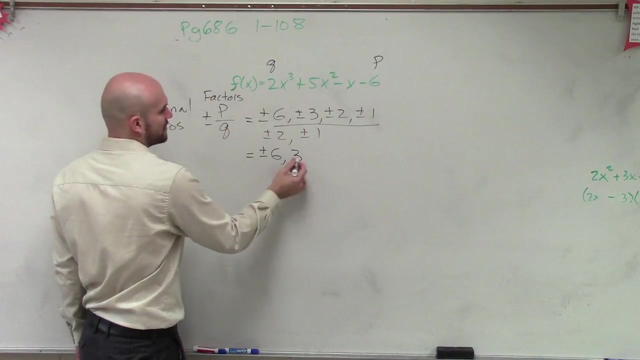 P is going to be your constant and Q will always be your leading coefficient. So now I just need to simplify this. Well, so what I'm going to do is I'm just going to start this in descending order. So 6, plus or minus 6 over 1 is 6, plus or minus 6 over 2 is 3.. 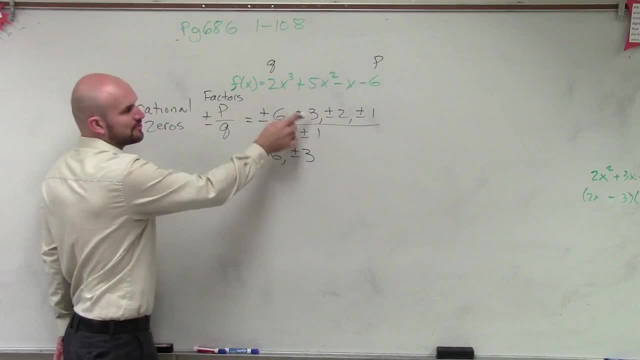 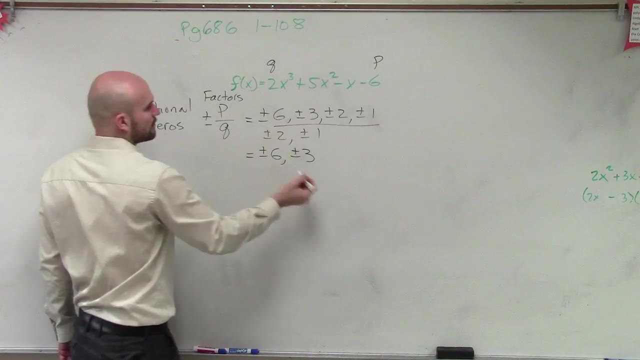 Now I don't need to do 3 over 1 again, because 6 over 2 gave me 3, right. So now I can just move on to 2 over 1.. So plus or minus 2, comma, if I did 2 over 2, that gives me 1.. 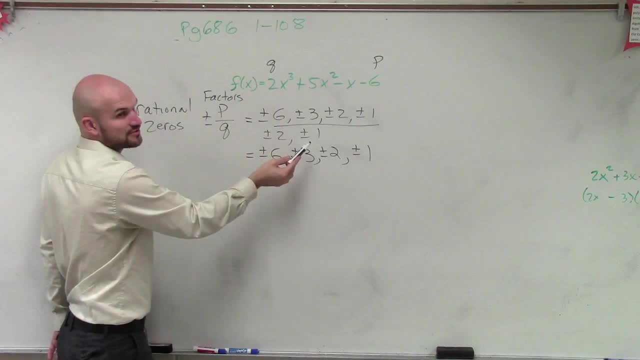 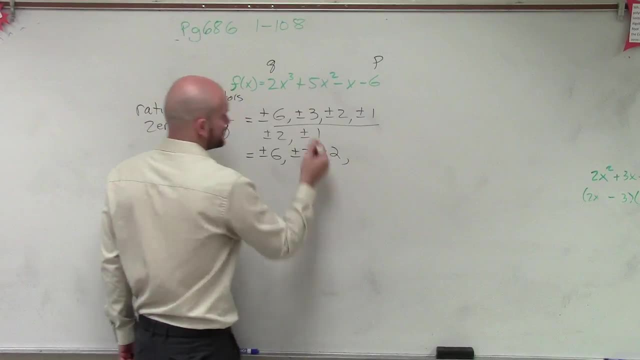 And then that means I don't have to do 1 over 1 again, because I know that answers 1,. right, I'm reading. I'm going to get to the fractions. Oh, I guess I could have done 3 over 2 would have been next actually. 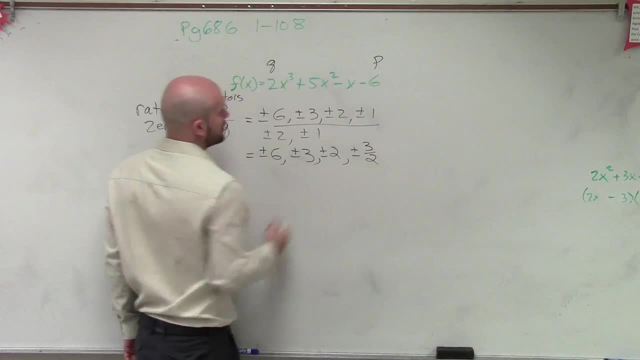 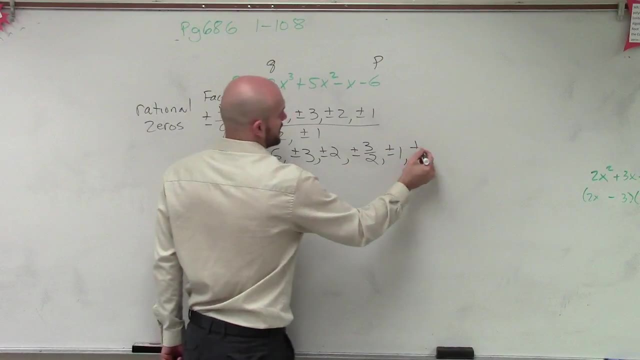 You're right, 3 over 2.. So 3 over 2 would have been your next fraction. right, There you go. Then plus or minus 1, then do 1 over 2, plus or minus 1 half.